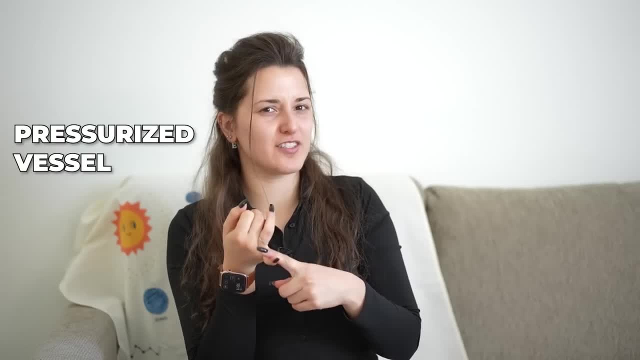 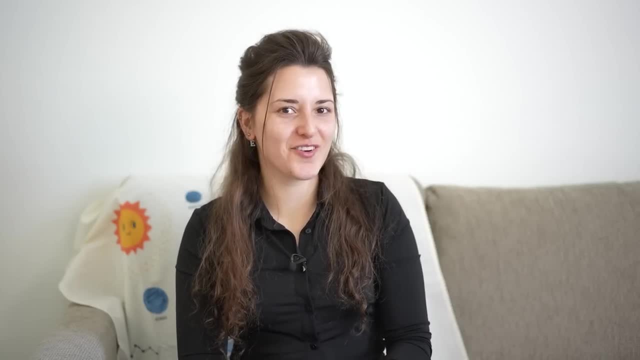 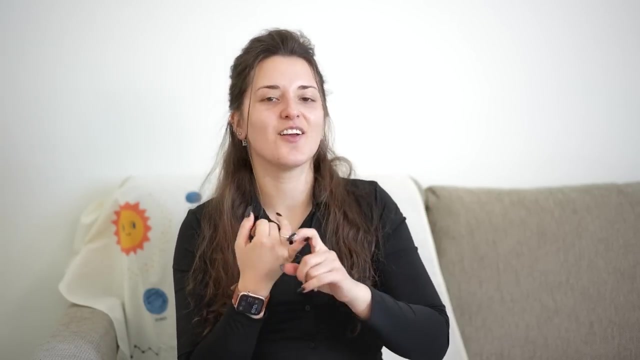 Hmm, CANDU reactors, pressurized vessel heavy water. what on earth are these reactors? Hey, there, it's Elina, your friendly nuclear physicist, and today we are discussing about CANDU reactors. We are going to be splitting this video into the following six categories. What is a CANDU reactor? 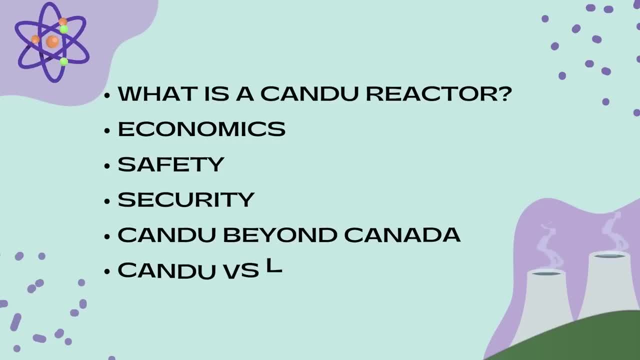 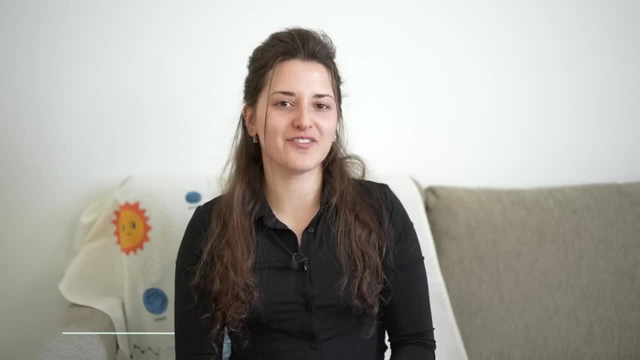 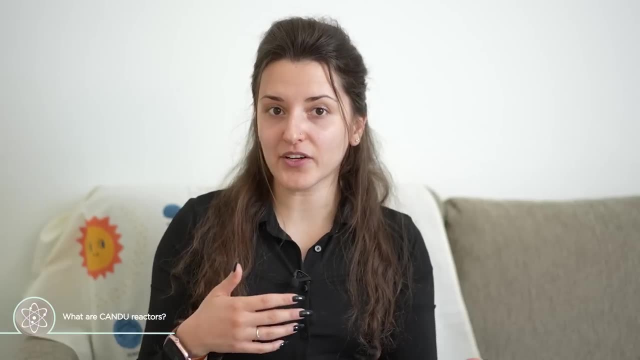 Economics, safety, security, CANDU reactors beyond Canada and CANDU versus light water reactors. Without further ado, let's get into it, Starting off by defining the abbreviation CANDU. it stands for Canadian Deuterium Uranium Reactor and it has a major similarity and a major difference compared. 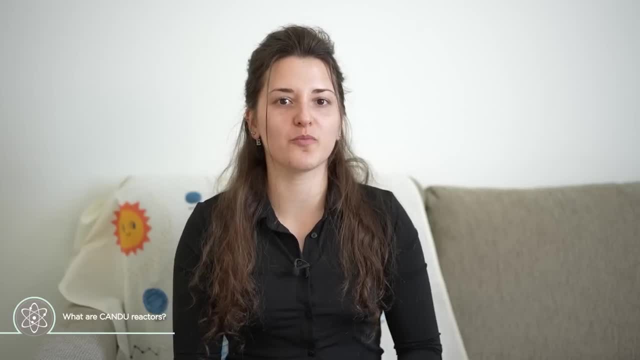 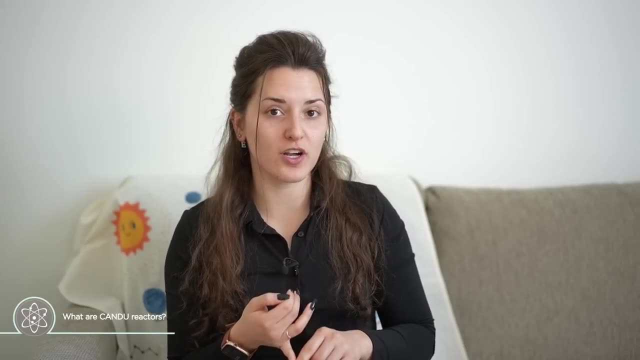 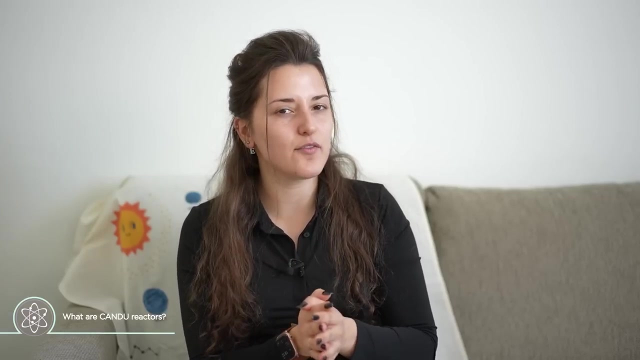 to the typical light water reactors that are used in Europe and USA- not just USA- in Europe and around the world. These are the fact that it's a pressurized vessel, similar to the light water reactors. However, the moderator and coolant of the CANDU reactors is heavy water. 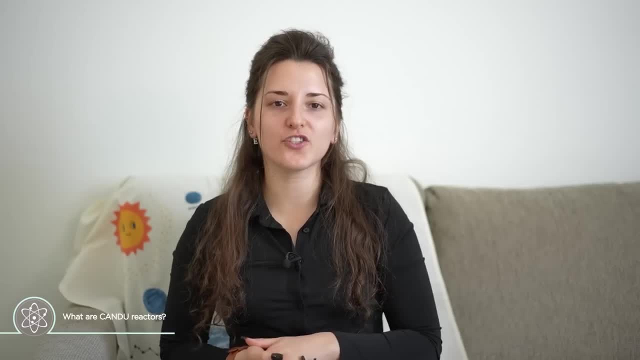 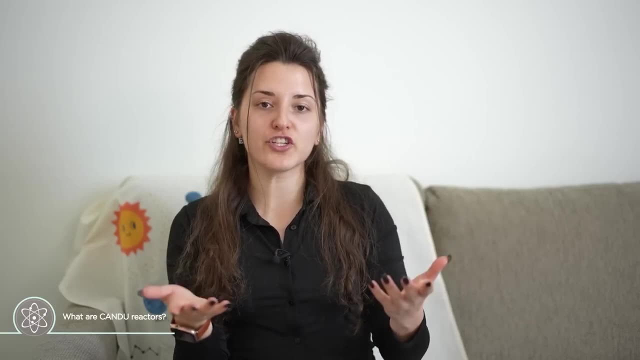 And we're going to get into what that means in a while. The principle of operation of a CANDU reactor is very similar to a typical light water reactor, meaning that we have a nuclear fuel fissioning inside the core, where neutrons are heating. the uranium fission is happening. 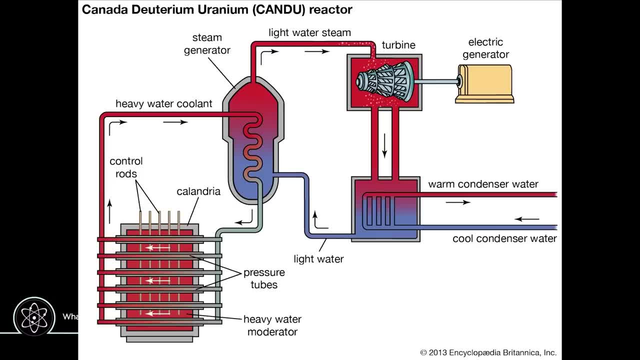 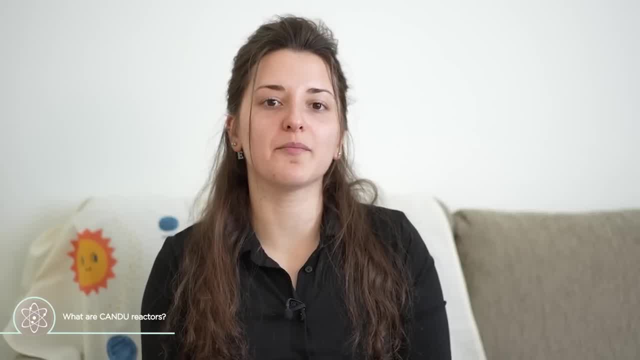 the atoms are split, energy is released, water is turned into steam, the steam turns steam turbines that then go and produce electricity. However, as I mentioned, the main difference of the CANDU reactors is the fact that they use heavy water. their coolant and their moderator. Heavy water is basically similar to regular water, with a difference that instead of hydrogen, there is deuterium, which is basically a proton and a neutron forming an atom together, and makes it heavier and denser than regular water. 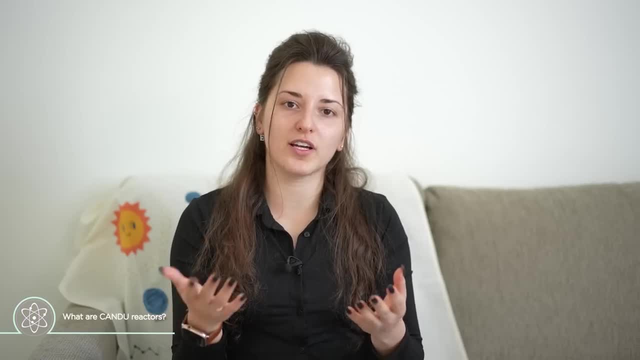 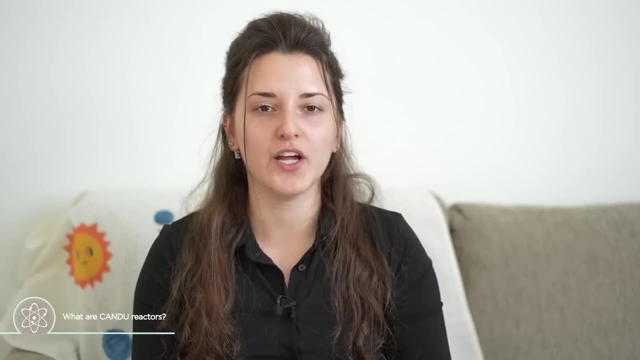 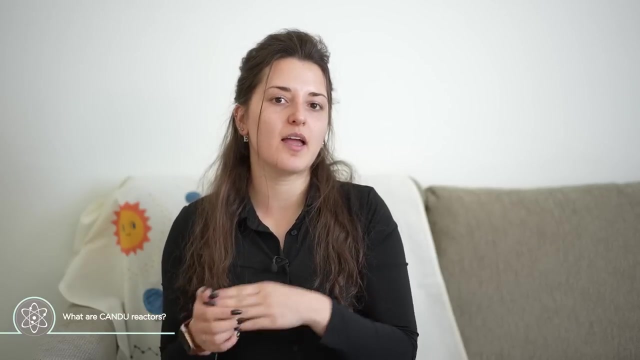 Hence that's why it's called heavy water. Deuterium water, or deuterium oxide, has a higher density and it is better moderator than the regular water. The natural abundance of deuterium in water is 156 over a million hydrogen atoms, making a concentration around 0.015%, which is quite low. 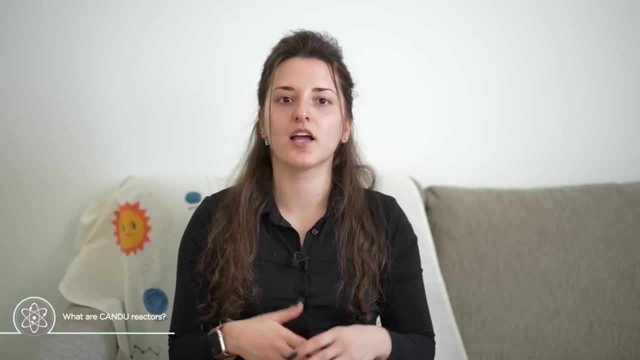 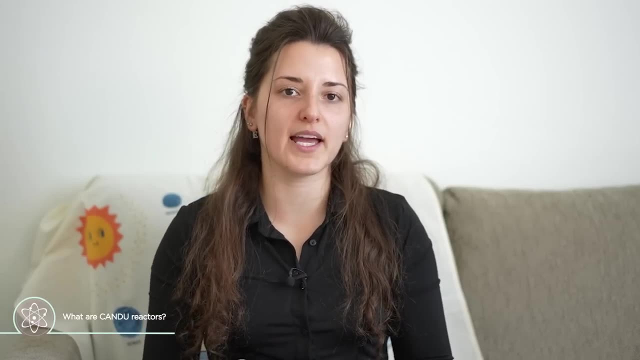 So typically, heavy water that is used for CANDU reactors is not only occurring naturally, since its concentration is so low, but it's actually produced from regular water, either by electrolysis or a chemical exchange of hydrogen into deuterium atom. These processes 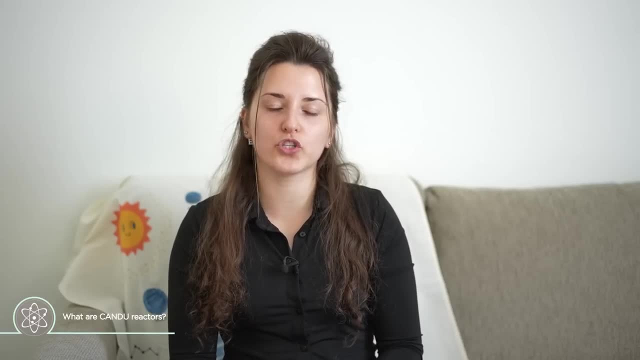 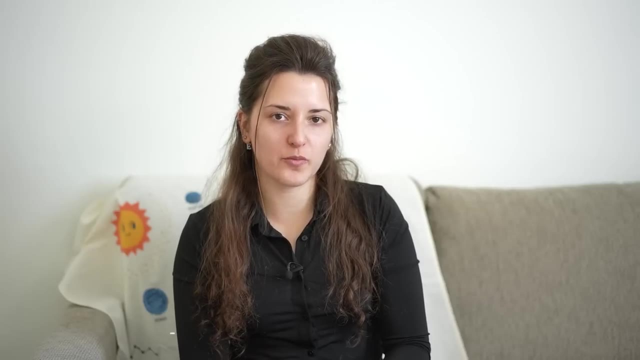 are cost effective and produce high purity heavy water, which is necessary for the operation of CANDU reactors and for efficient moderation of neutrons. So, moving on to the economics aspect of this type of reactor, and here we have several advantages and disadvantages, And already 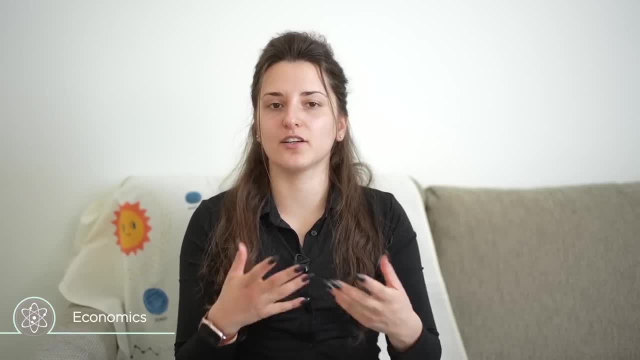 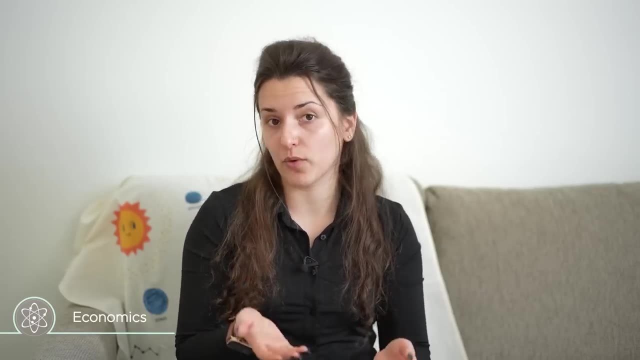 disadvantage was mentioned in the previous section is the fact that CANDU reactors require heavy water, meaning that, first of all, it is more complex to produce it instead of using regular water And, second of all, the production itself is costly and adds to the total cost of the operation. 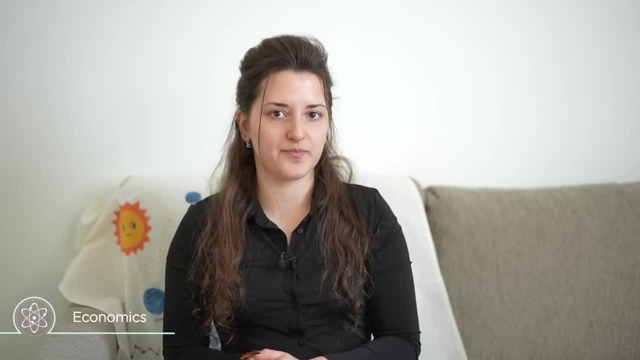 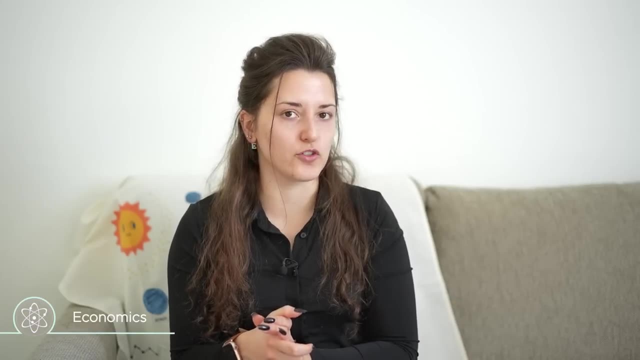 of the reactor and hence the cost of the reactor's function. So there are two main reasons why it's hence the electricity price. However, you might ask, if it is more expensive, then why use heavy water at all? Why not use regular water than, like in light water reactors? Heavy water has an 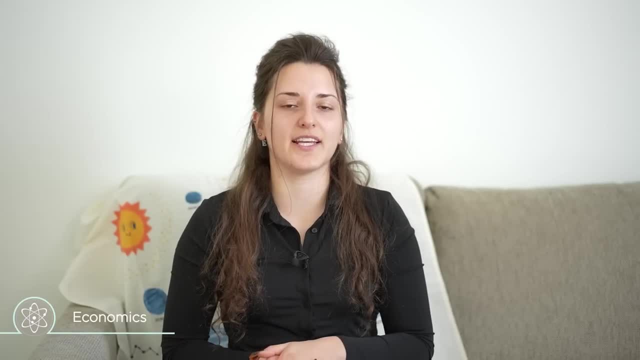 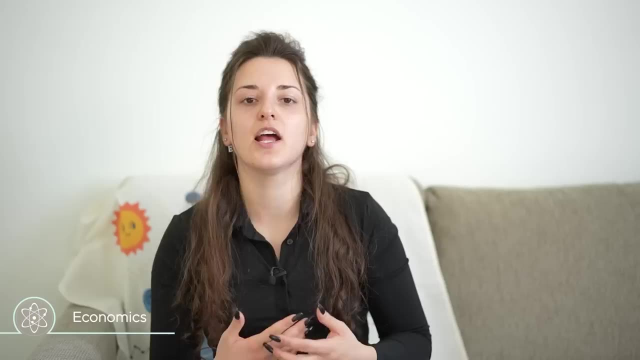 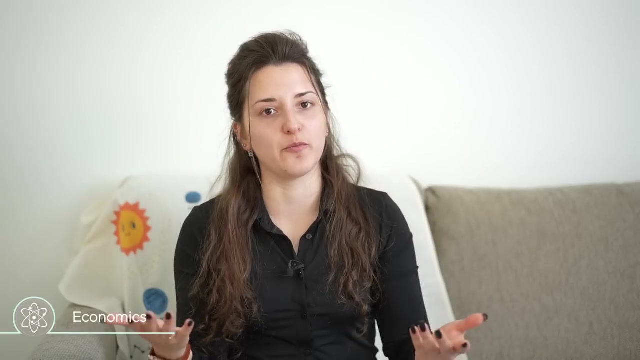 advantage- and this is the reason why it was chosen by the Canadian authorities- is the fact that, since it is a better moderator, meaning it slows down neutrons more efficiently than light water does, means causing more fusions. it can actually be used with natural uranium, meaning that in 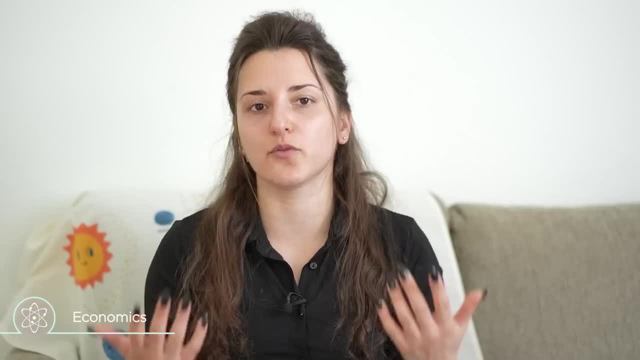 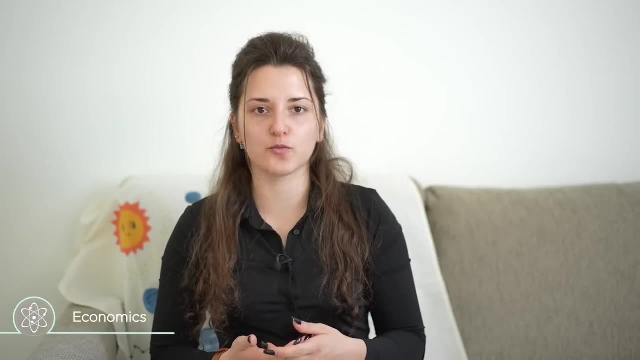 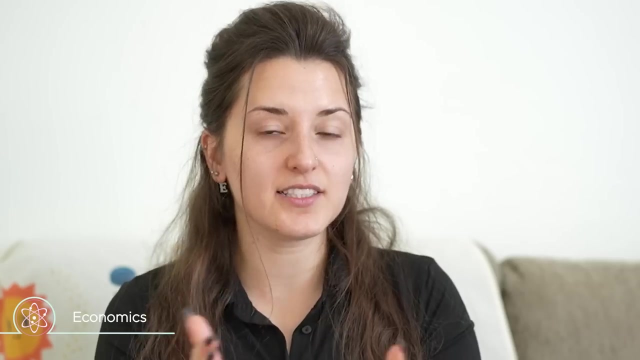 can-do reactor types. the fuel doesn't necessarily need to be enriched. It can be used in its natural form, as in uranium-238, which is not efficient to be used in light water reactors and would not have a sustainable fission chain reaction if it was to be used in those type of reactors. Hence even 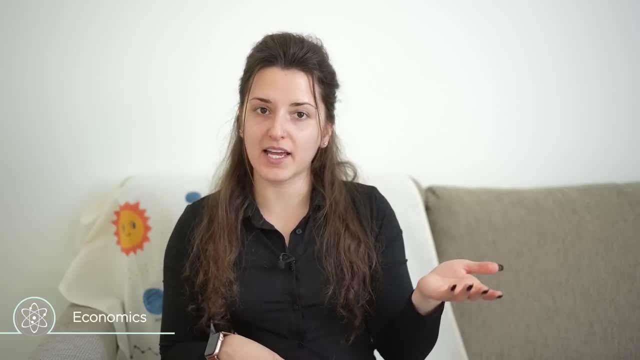 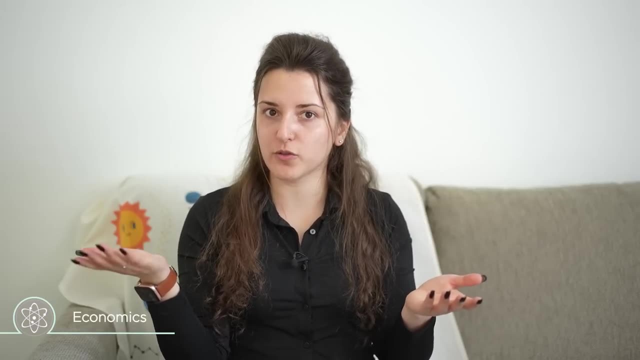 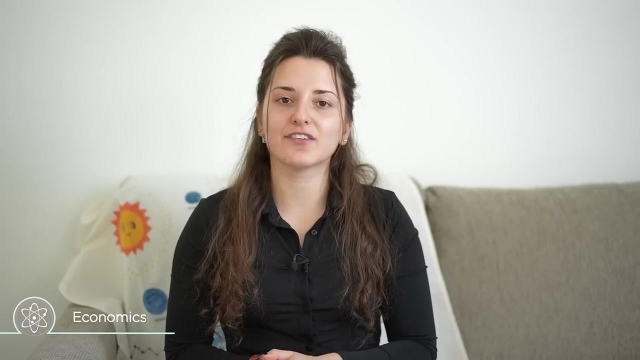 though we do add a cost and a complexity factor by employing heavy water, we also reduce cost and complexity by the fact that enrichment in uranium fuel is not necessary. Another major advantage of can-do reactors and their design is the fact that they can be refuelled. while still in operation. They have quite a different design from the typical light water reactors and the fuel rods are basically horizontal instead of the usual vertical that we have seen in pictures in the past, and that allows the fuel rods to be removed individually and replaced with new fuel rods while the reactor is still under operation, reducing 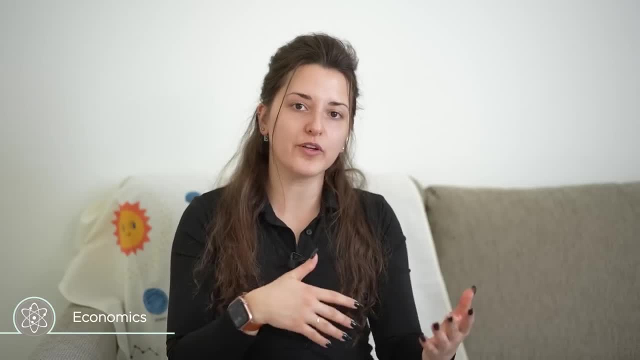 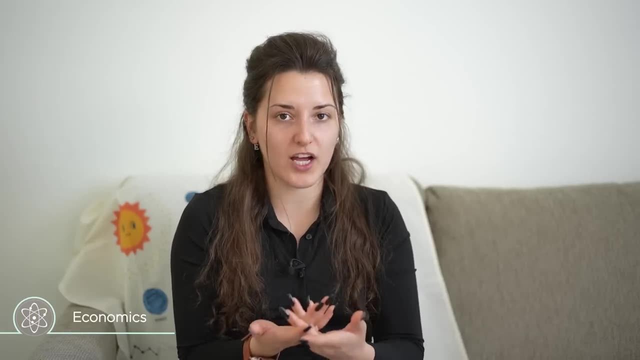 the downtime, so the time that the reactor needs to be shut down, refuelled, checked and went back into operation, meaning that the cost of the electricity production, the cost of the maintenance itself, is much lower and it is a much more efficient process to do so. However, by having 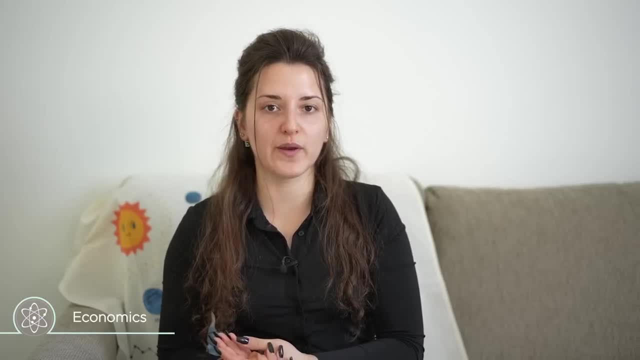 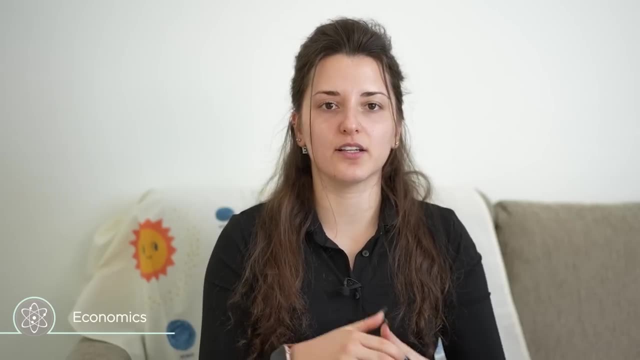 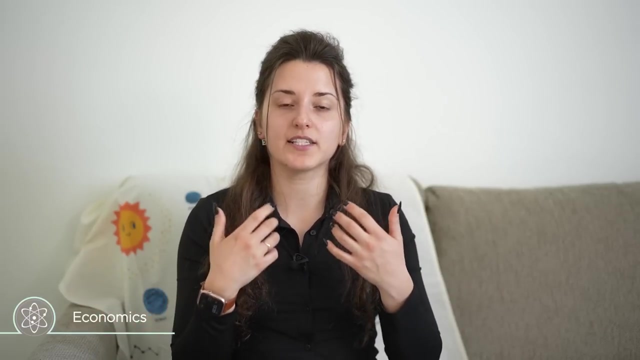 this advantage of online refuelling of the reactor adds to the complexity of the design itself of the can-do reactors, which of course might enhance the cost of constructing the reactor. But, as we said, while in operation the online refuelling is a very good advantage on the cost of the 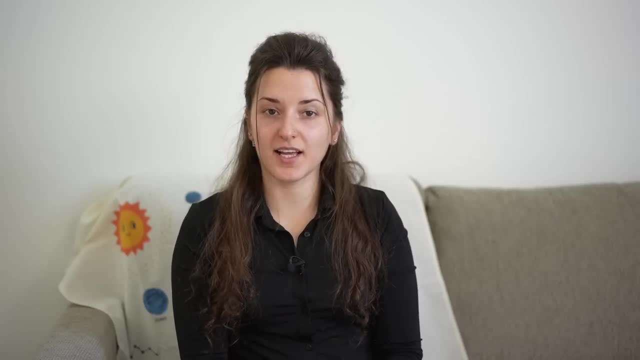 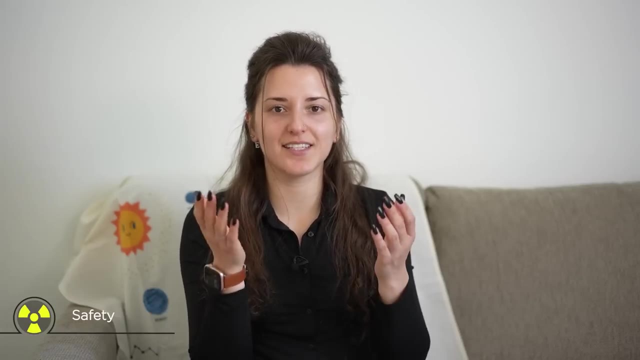 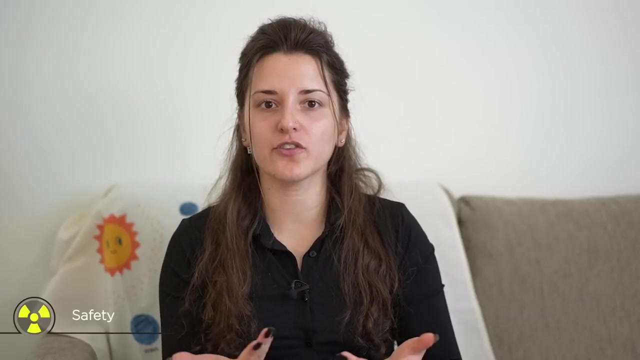 electricity price itself. Moving on to our next aspect, and we are going to discuss safety. Safety is a major issue in all nuclear reactor types and can-do is no exception. So, regarding to the safety aspect of the can-do reactor, here it is important to mention that can-do, since it's using heavy 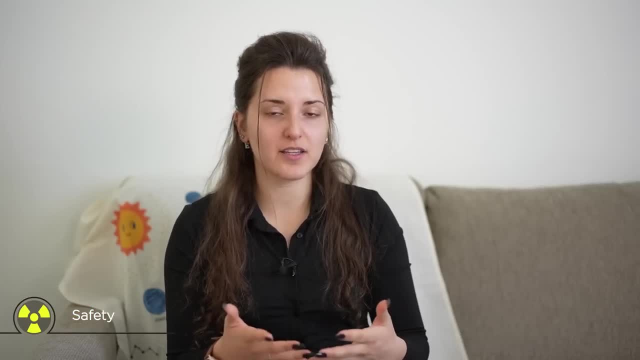 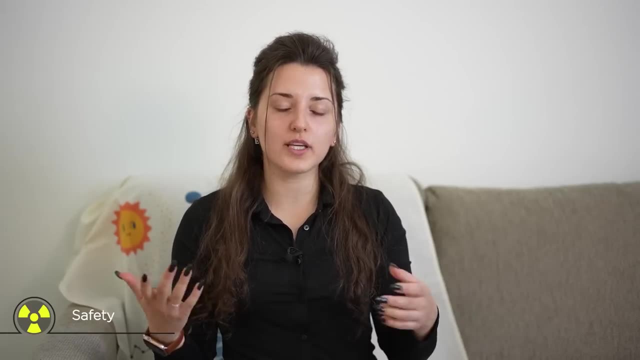 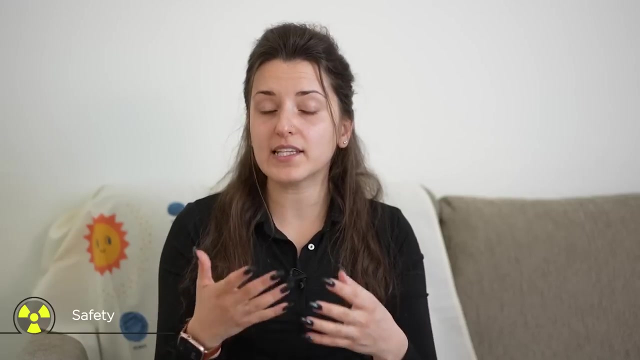 water is actually safer in various ways. For example, in the case of the can-do reactor, the water is less reactive than regular water, is meaning that it is less likely to cause a meltdown or even a chemical reaction between the coolant moderator and any other part of the reactor. in 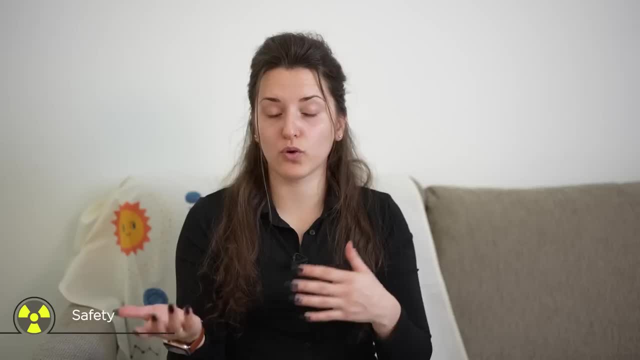 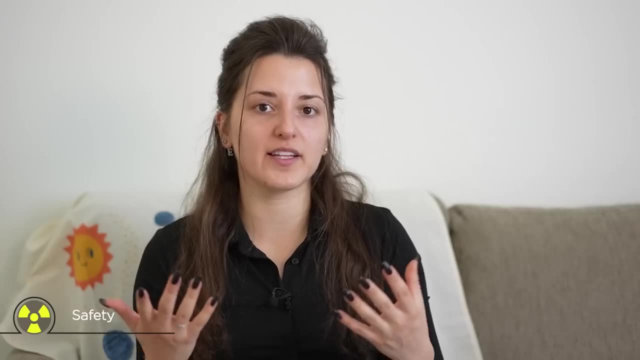 case of an accident. Additionally, can-do reactors, similarly to light water reactors, use a pressurised system, meaning that the coolant is under high pressure for it to prevent boiling, which is a good safety feature that the reactor has, and it is also a very efficient system for the air-conditioning. 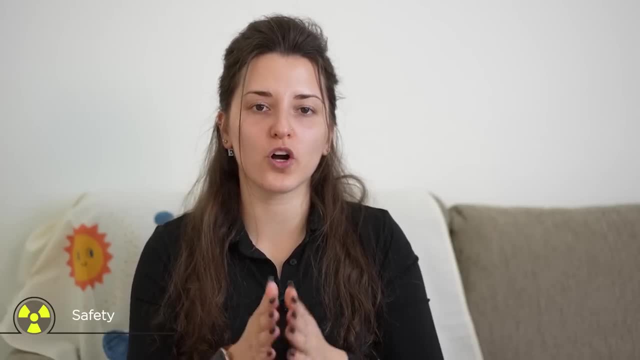 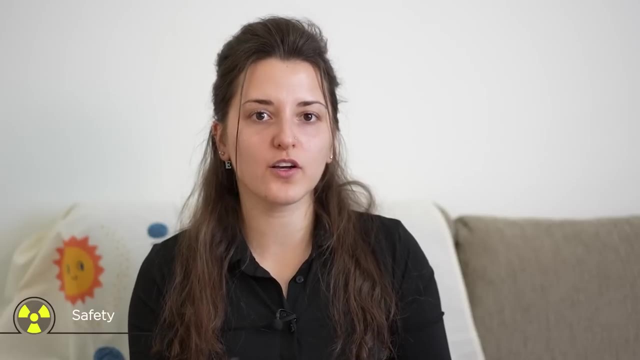 of the reactor. So, for example, if water is too hot, the reactor can explode, and the air-conditioning is also better in order to contain the radioactive material to not be released into the environment in case of an accident. Regarding the online refueling of the Cantu reactors- and here a loss, 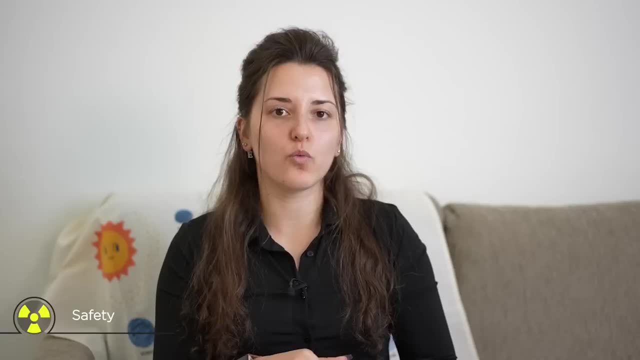 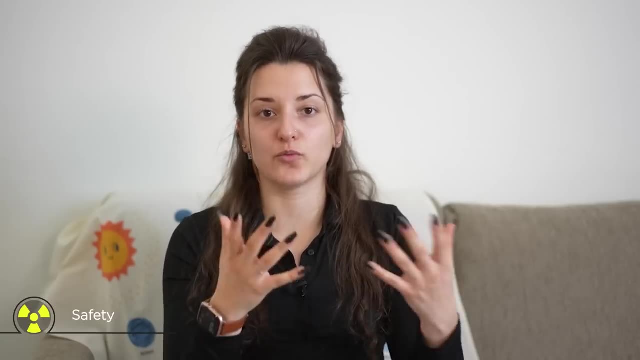 of coolant. accident, or else called lock-up, might occur while the fuel rods are being removed from the reactor. The coolant actually might leak out in case of an accident and radioactive material might be released into the environment. However, there is a lot of safety features in place to 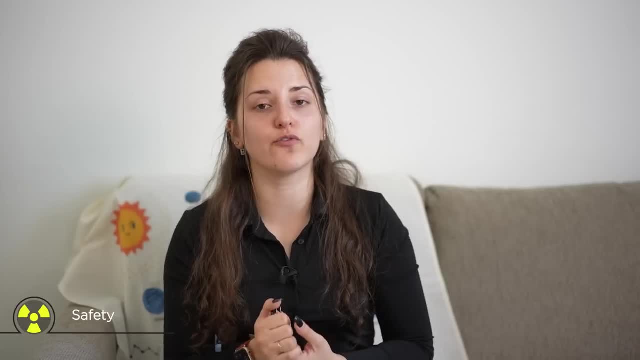 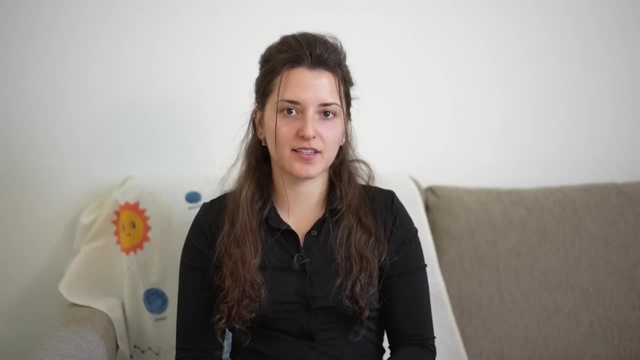 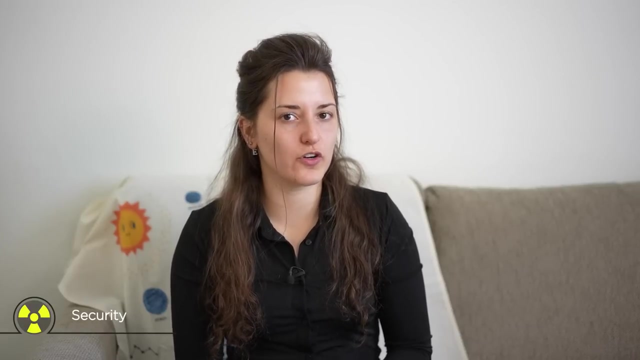 actually account for that, and the possibility of such an accident occurring while the refueling is ongoing inside the reactor is very low. Moving on to the next aspect that we're going to discuss, and this is safety. Here, Cantu reactors have several advantages over light water reactors and 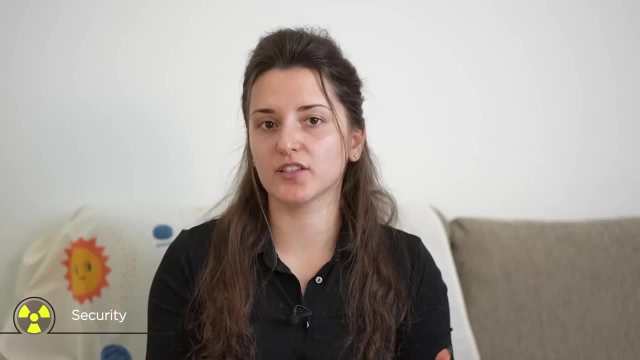 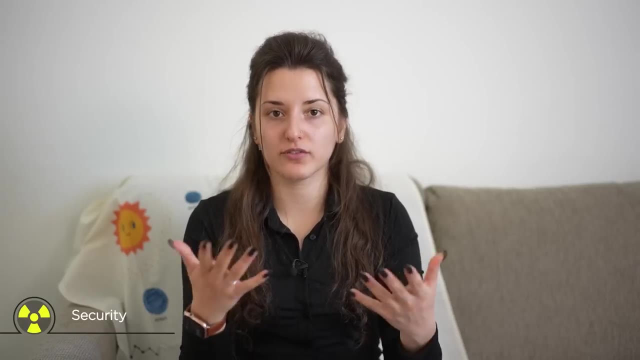 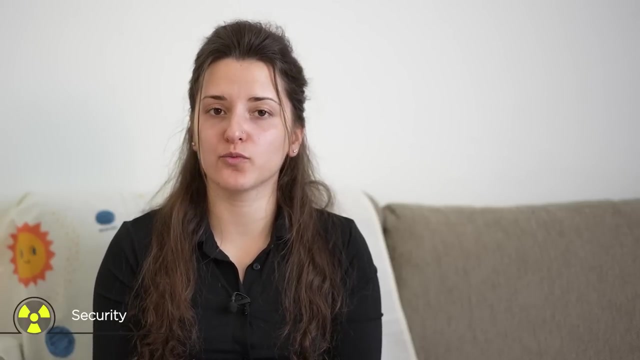 one of them is the fact that they can use a wide variety of fuel in order to operate and produce electricity. This, for example, means that instead of natural uranium, which we already explained these advantages over enriched uranium, they can also use a fuel that comes out of light water reactors and being reprocessed, So, basically, they can also use spent nuclear fuel. 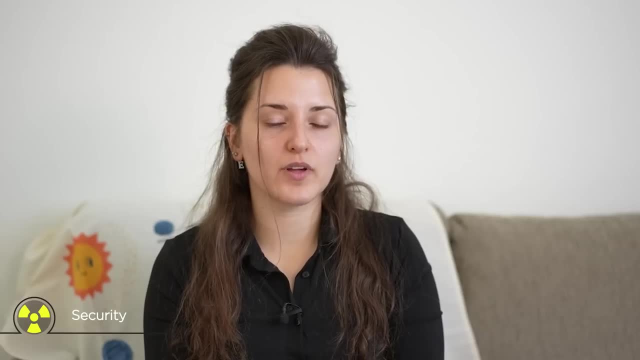 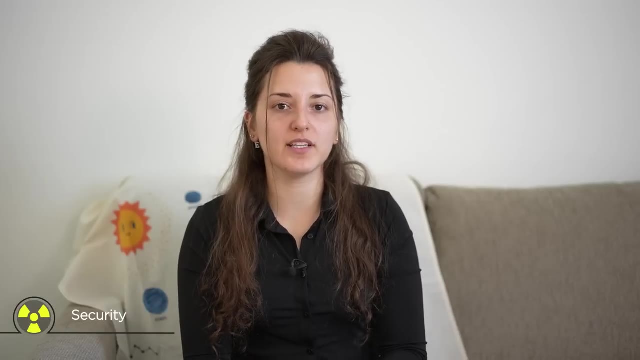 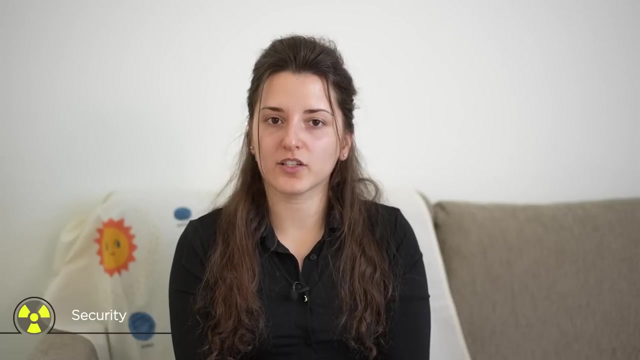 coming out from light water reactors. So this makes Cantu reactors less dependent on a single fuel source and less vulnerable to supply disruptions in case fuel is not able to be delivered or enrichment is not available. This is also possible in the countries that do enrichment of uranium Additionally, Cantu reactors. 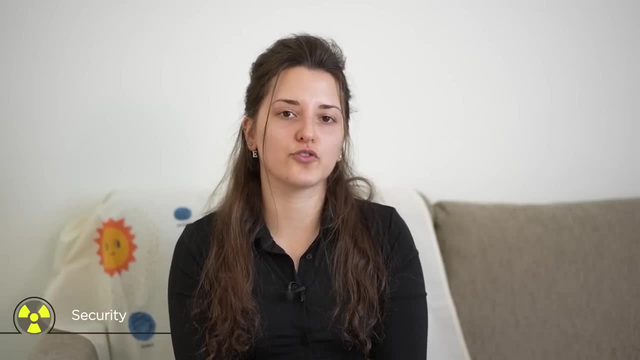 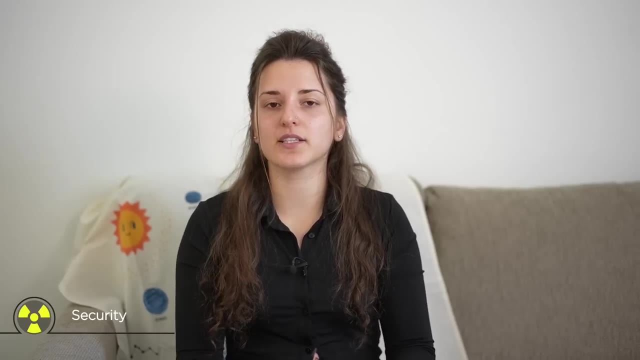 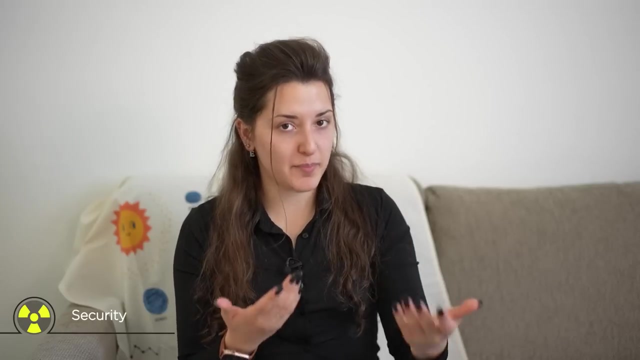 do not produce weapons grade plutonium like light water reactors do, which makes them less interesting for proliferation issues and concerns How they do that is. the fact that they use deuterium water actually aids in that, because deuterium water besides being a, let's say, better moderator it. actually has the ability to also absorb more neutrals than the water that is produced by the regular water does, meaning that it leaves less neutrons for the fission products to be turned into plutonium. hence less plutonium is produced inside the reactor, inside the fuel and additionally. 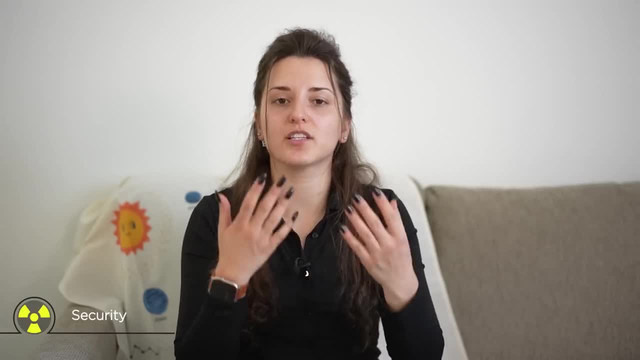 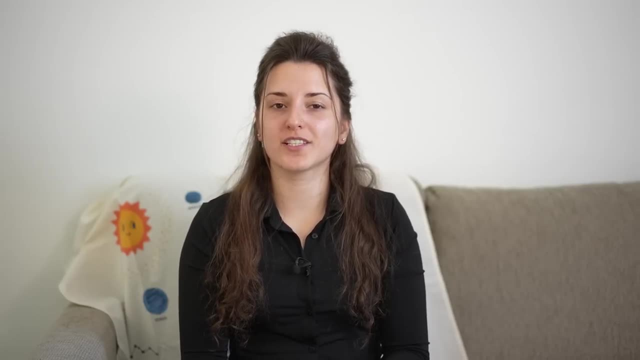 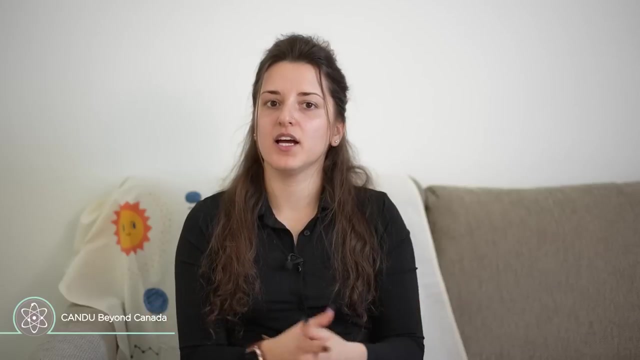 Cantu reactors operate at lower temperatures than light water reactors, which is an advantage, again, over producing less plutonium inside the vessel. So, moving on to the most interesting aspect in my opinion is why aren't Cantu reactors then used around the world if they have such advantages that we already discussed in the previous points? So Cantu reactors were. 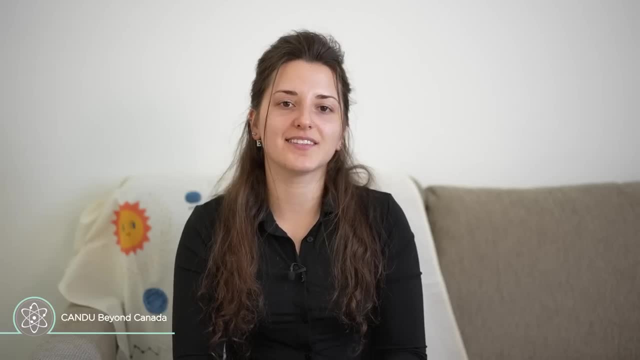 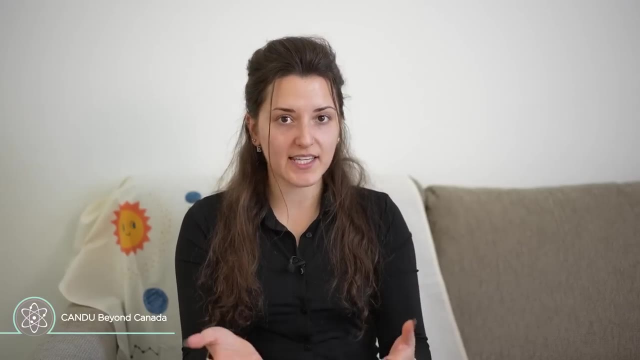 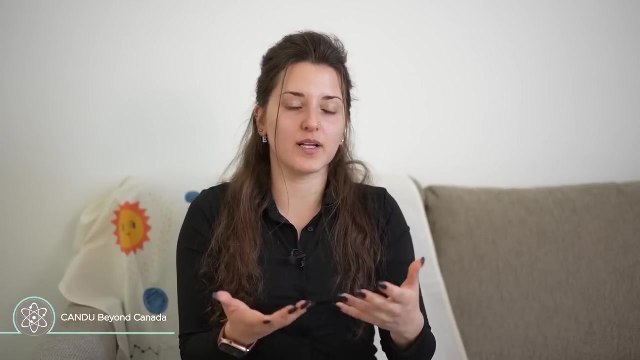 developed in Canada, hence their name. and the expertise for the Cantu reactors in Canada is very advanced because people there have been working with these reactors for decades. they have been building them, they know exactly their problems, how to fix them, and they're very good at doing that. hence they are not, let's say so, interested in other types of reactors and they 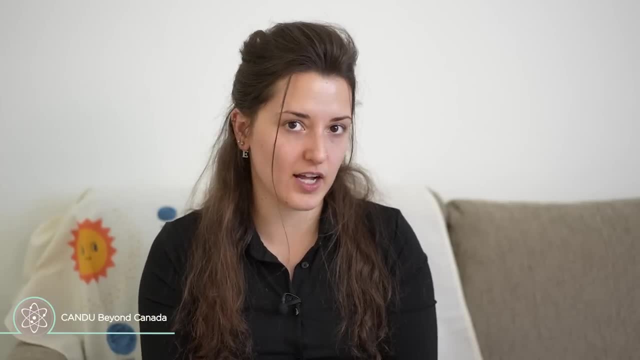 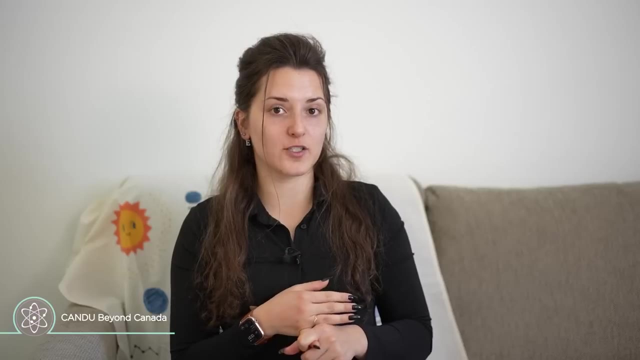 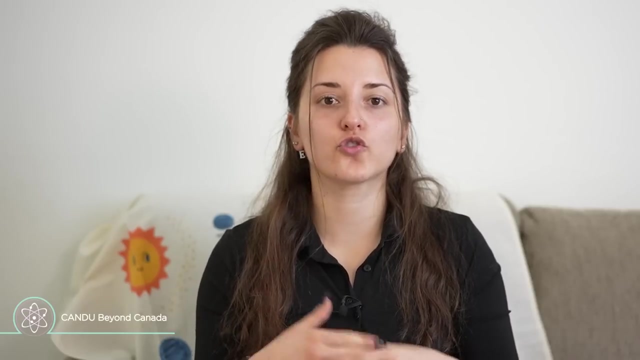 are very interested, however, in selling this technology in other countries. it might come as a surprise, but Cantu reactors do exist in other parts of the world as well. for example, Romania has purchased two Cantu reactor types. so has Argentina and China. other countries have also tried to use the technology, such as: 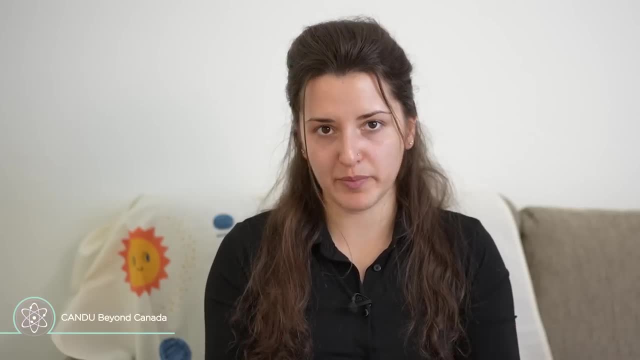 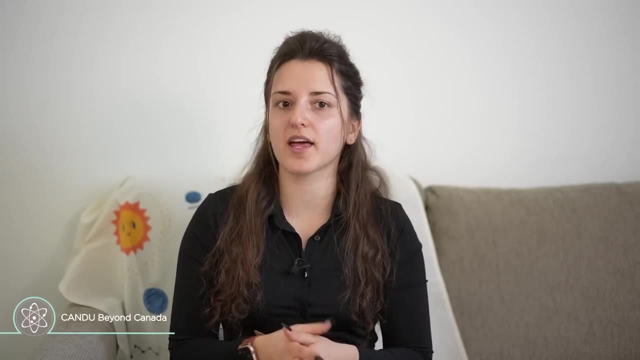 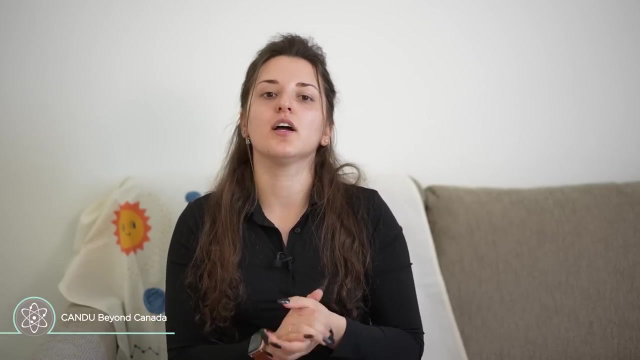 India, Pakistan, South Korea. however, they have never actually built a Cantu reactor. so these countries, even though they have Cantu reactors, they don't seem to be doing very well with them, and that's stems from the fact that the expertise are much lower in Europe and Asia when it comes to Cantu. 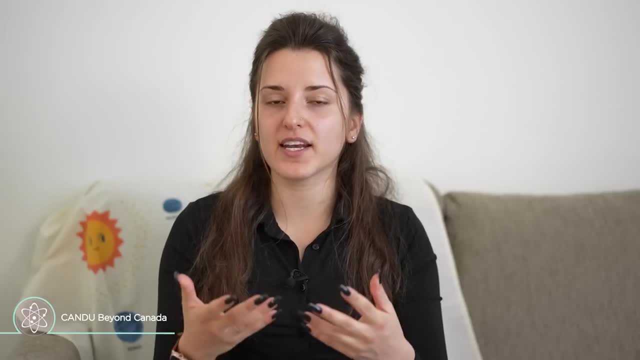 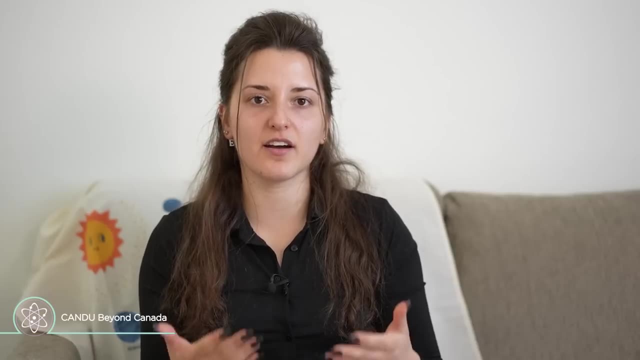 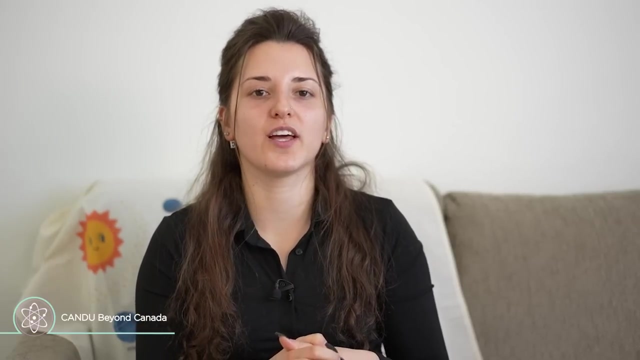 designs. compared to light water reactors, therefore, they are not really so popular when it comes to being, let's say, built and delivered around the world, as they are very popular in Canada. that is the main reason why the Cantu reactors are, let's say, kind of limited to the borders of Canada. however, they are very widely used within the country and, as 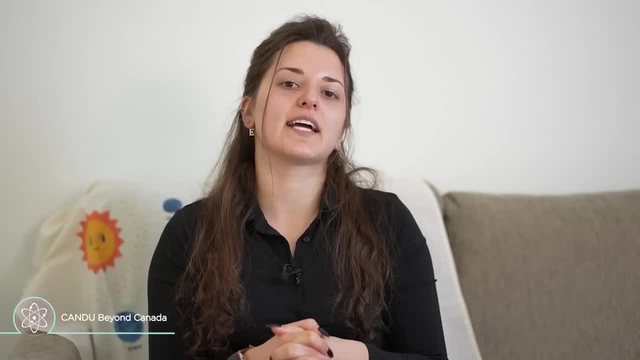 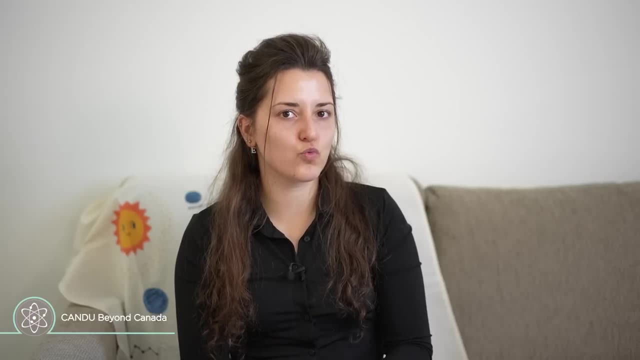 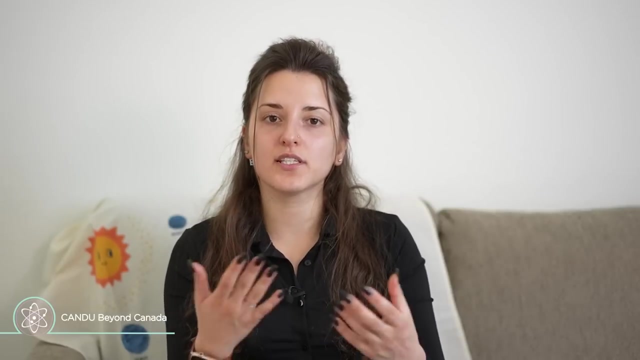 you already mentioned, the expertise and the knowledge that the Canadian authorities, nuclear authorities, have over this design is superior. then one might ask why develop a Cantu reactor design in the first place and not use a light water reactor even in Canada? so it is interesting to point out that Cantu reactors are basically chosen in Canada because of the Canada's natural resources. so Canada is abundant in natural uranium, which is exactly the fuel that use for their reactor types, as well as quite high in abundance of heavy water. Therefore, it is perfect for them to design a reactor type that actually uses both of. 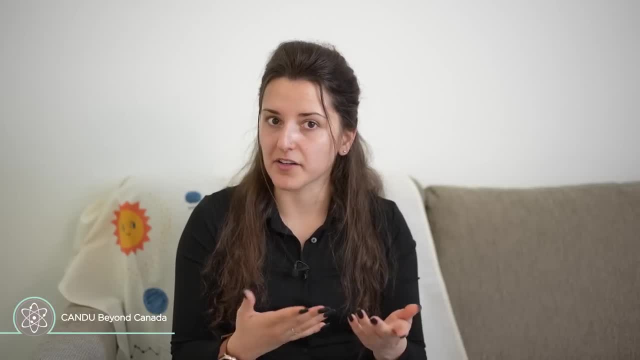 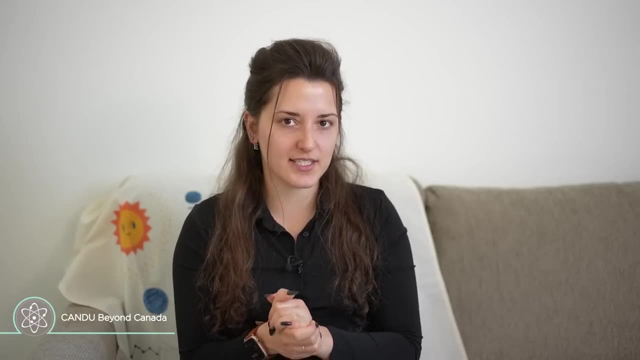 their natural resources. That is why their design is quite popular in Canada, but might not be so attractive in other parts of the world that don't share the same abundance in natural resources as Canada does. So, moving on to the last point, and that is so, which one is better? 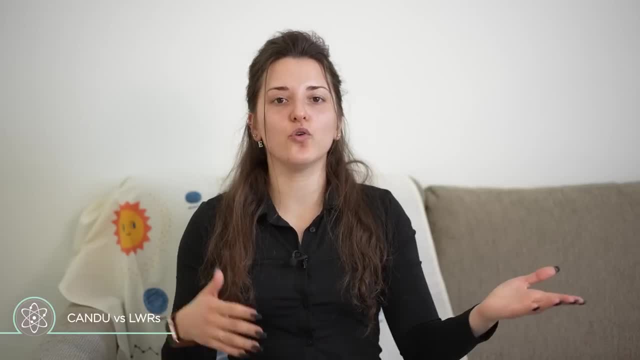 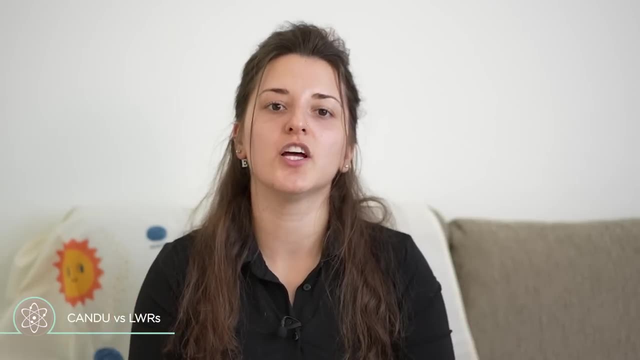 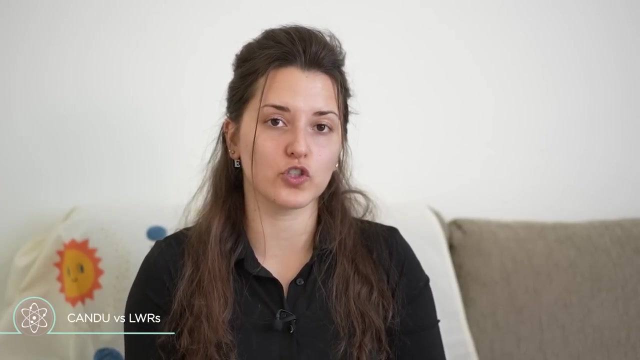 Which one should we choose? Which one is cheaper, Is it can-do or is it light water reactors? So here, of course, the price and the economics, which is the major reason to basically build a reactor design. it really depends on the location where the reactor is going to be. 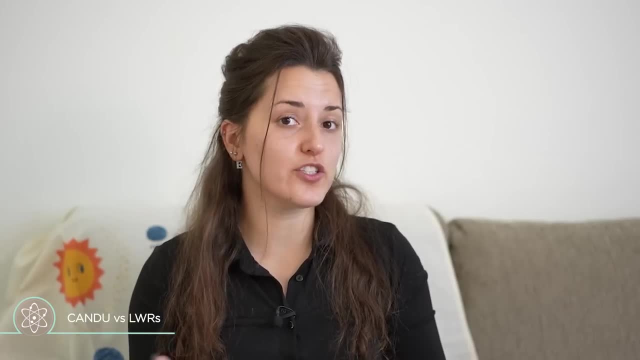 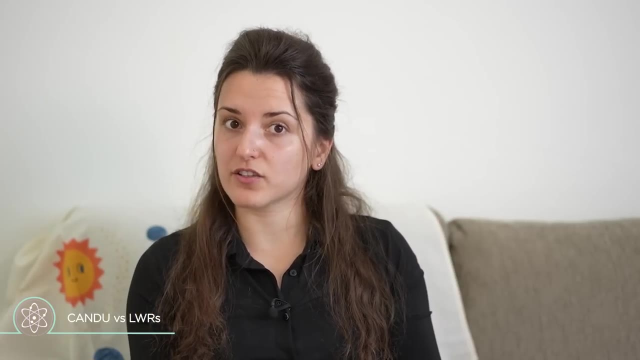 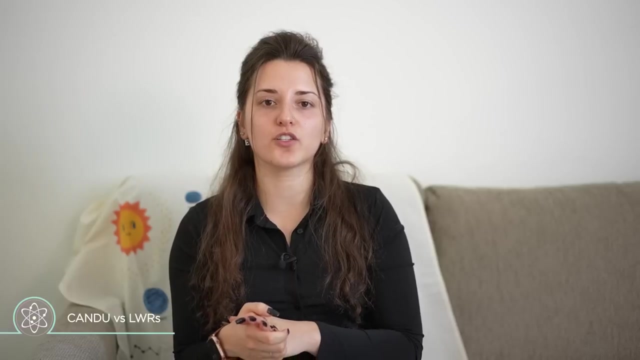 built, the size of the reactor, as we already mentioned the resources of the country that will host the reactor itself. However, there are several advantages and disadvantages And we're going to sum them up here. The can-do reactor type has several advantages over light water reactors, and that is the 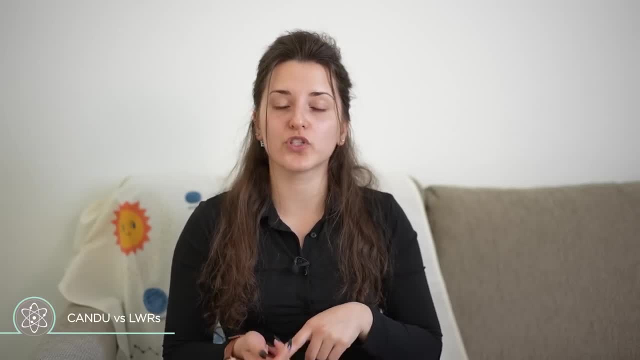 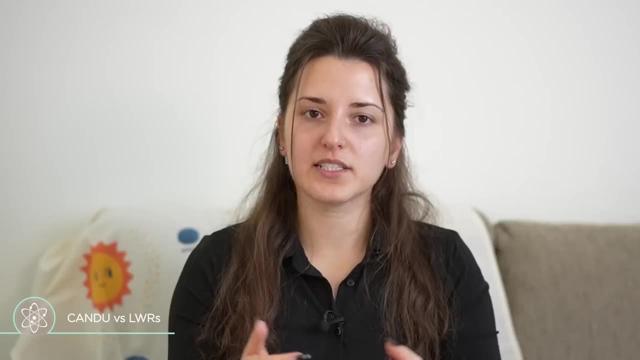 fact that it uses natural uranium as a fuel, which reduces the cost of enrichment, simplifies the process of basically producing fuel for the reactor as well, as it can use various fuel types as well as fuel that is being basically used in other reactor types, making 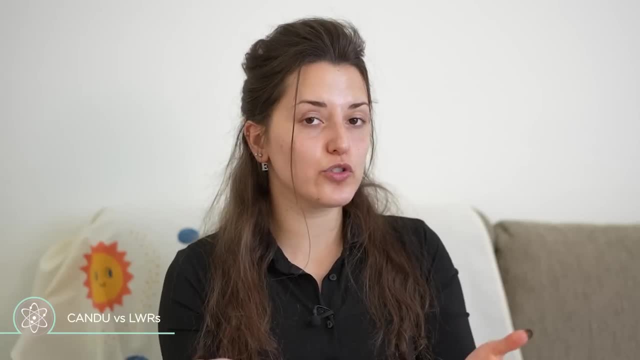 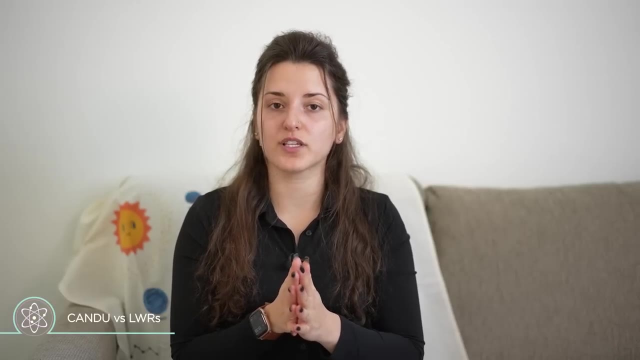 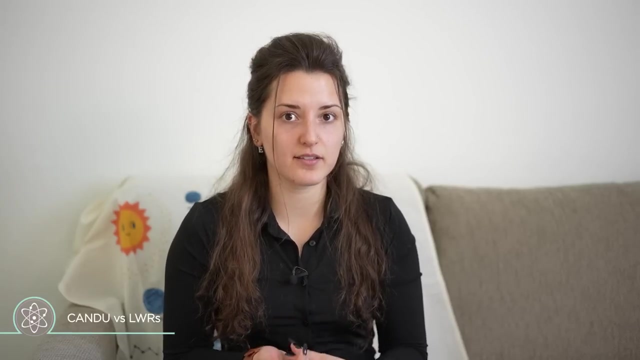 it even more flexible and potentially reducing the cost in the future if such technologies don't work. And the last advantage of the can-do reactor is the fact that it's being, as we said, refueled online. It reduces the cost of the downtime, let's say maintenance, and any kind of cost associated.